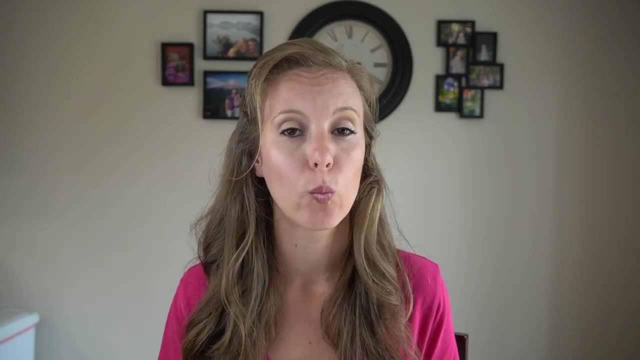 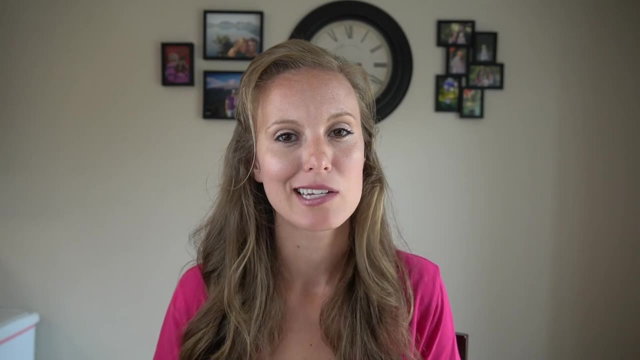 you do. As someone who manages to keep their home clean while working on my business for over 40 hours a week and having a two and a five-year-old at home with me full-time, I can tell you that the secret to having a house that is clean all the time has nothing to do with having extra time on. 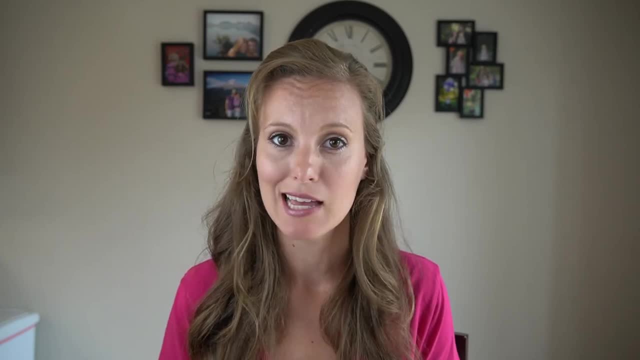 your hands. There are plenty of ways to keep your house clean. There are plenty of ways to keep your house clean. There are plenty of other things I could spend my time on instead of cleaning, and I am definitely not bored while trying to run a business from home with a two and a five-year-old. 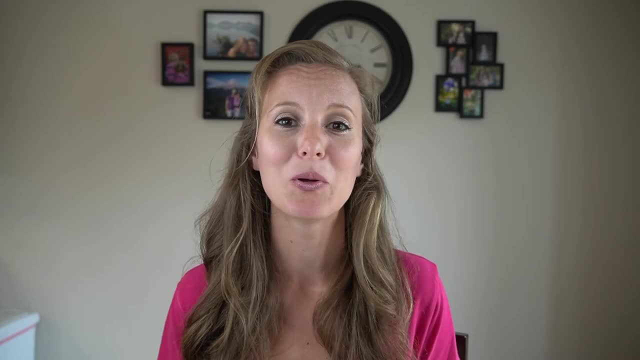 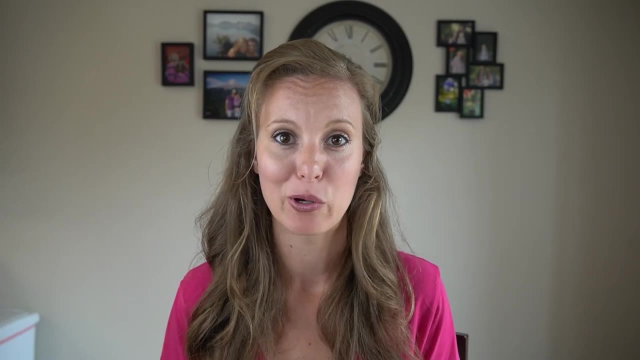 Although I have been asked both of those questions many times by people who are curious how I keep my house so clean. The reason I'm able to keep my house clean while running a business and having a two and a five-year-old at home full-time is because I know the seven secrets to keeping my 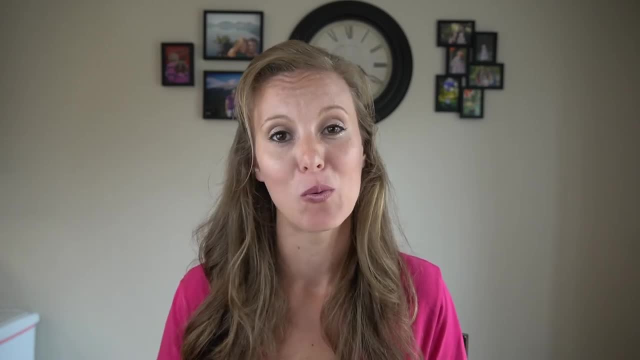 house clean all the time And in this video I am going to share them all with you. If we haven't met before, I'm Cassie with MakingTimeForGigglescom and I make videos all the time to help you. 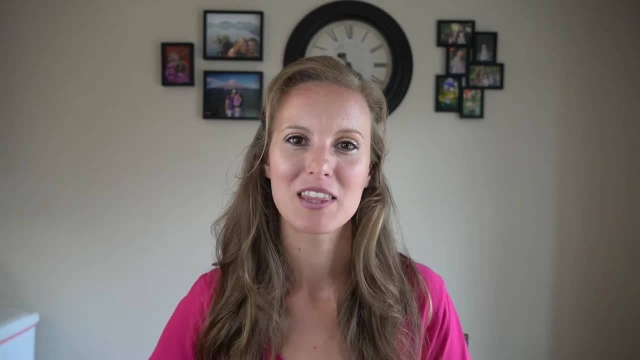 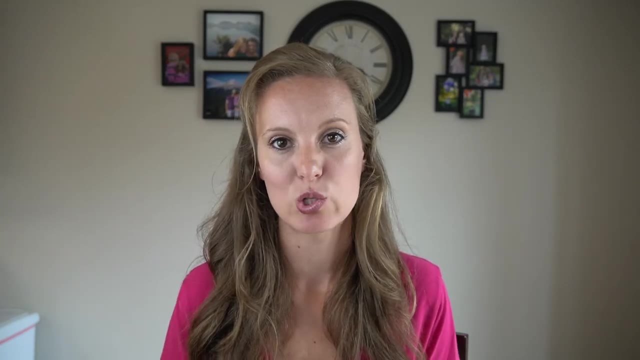 keep your house clean. This video is all about making mom life simple, So be sure to hit subscribe and ring the bell next to it if you would like to see more videos like this one. All right, let's get started. The first thing that people who always have clean houses do is they make their beds first. 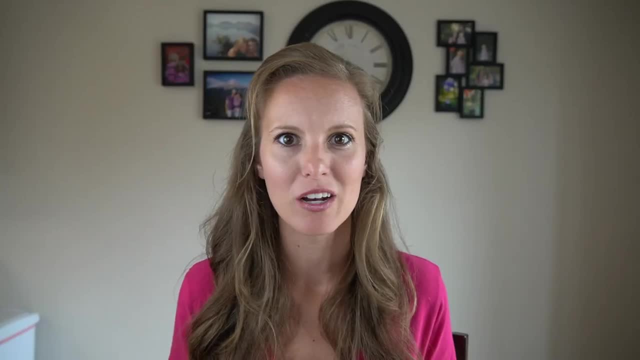 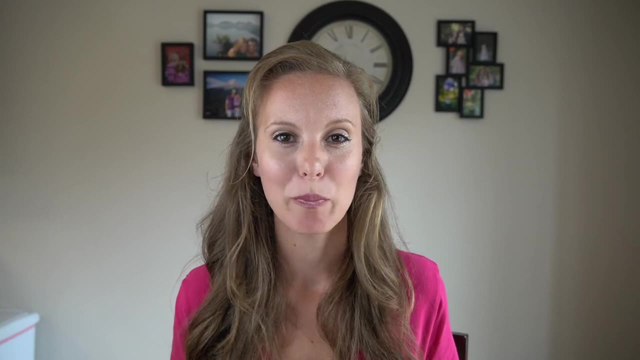 thing in the morning. I know this can seem like a simple thing and maybe a little bit of a waste of time when you have so many other things on your plate as a busy mom, but it can make a huge difference in how your house feels. Making your bed first thing in the morning helps your room. 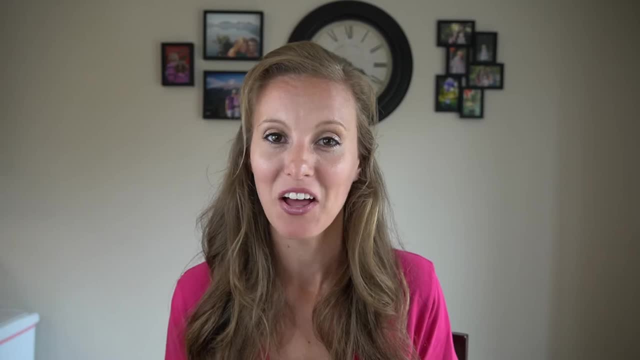 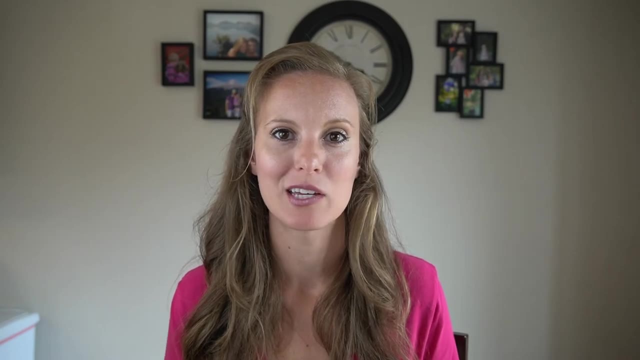 feel so much cleaner. It makes it much less likely that you will pile other things on your bed as you go throughout the day. It will teach your kids to make their beds in the morning and it allows you to check something off your list first thing in the morning. So if you aren't already in the habit, 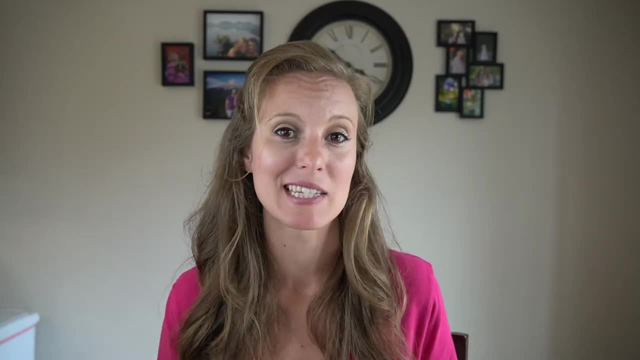 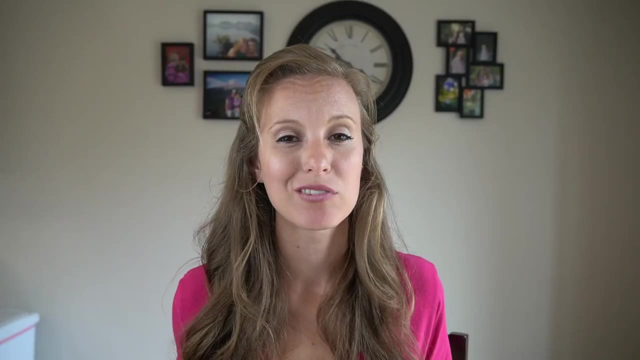 of making your bed every day. give it a try and see if you notice a difference in how clean your house feels. The second secret to having a clean house all the time is staying on top of the laundry. People who have clean houses all the time stay on top of the laundry with a simple 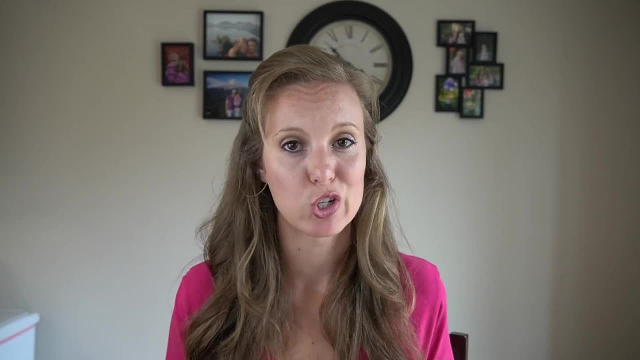 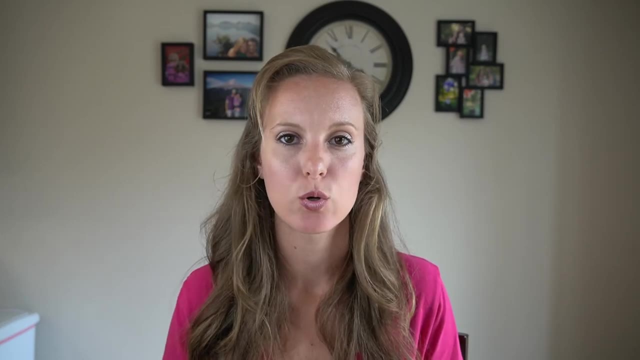 predictable laundry routine. Whether the piles of laundry in your house are dirty, clean or folded and waiting to be put away, it adds to the clutter in your home. Keeping your laundry under control will make a huge difference in how clean your house feels. I will put a link in the description. 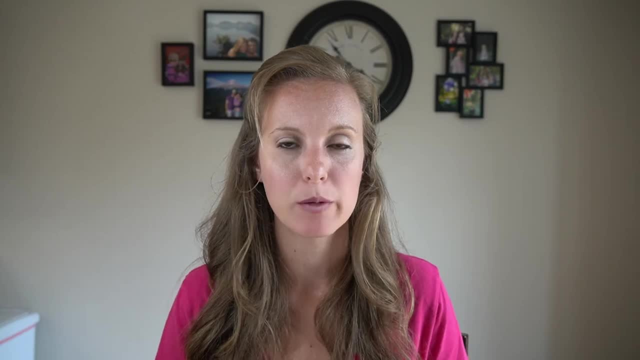 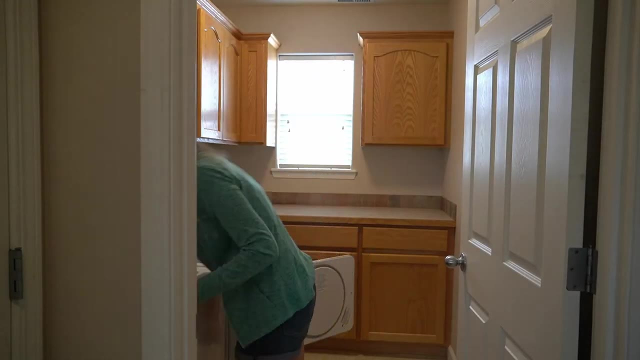 down below with a full article on how to solve the laundry problem and create your own laundry routine. but the biggest thing to remember when creating your laundry routine is to do one load of laundry every day, from start to completely finished, folded and put away The reason you. 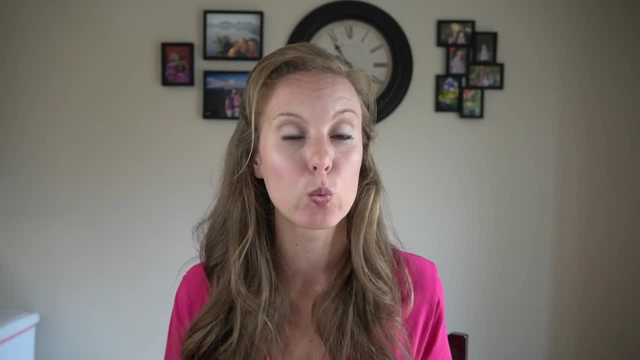 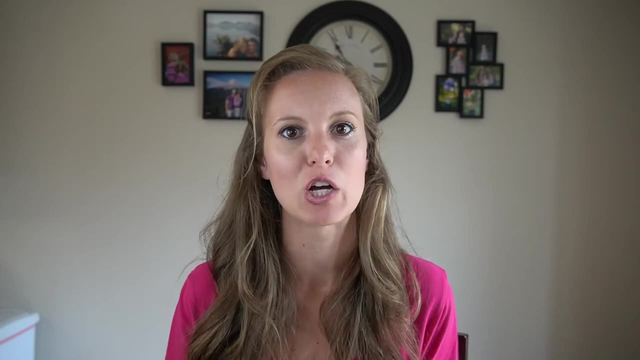 don't want to do laundry on only one day of the week is that it is really easy. at the beginning of the laundry day, You're just putting laundry into the washer and switching it over and starting another load of laundry, And when you do your laundry this way, before long you will have a 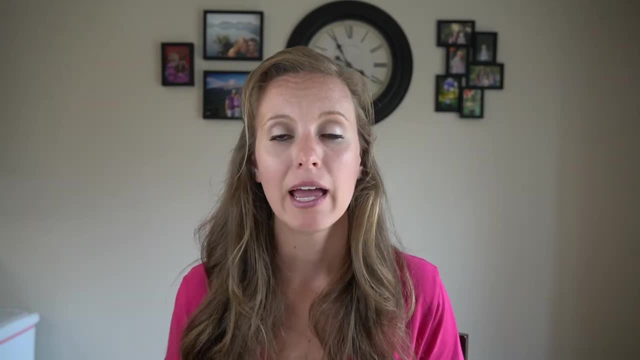 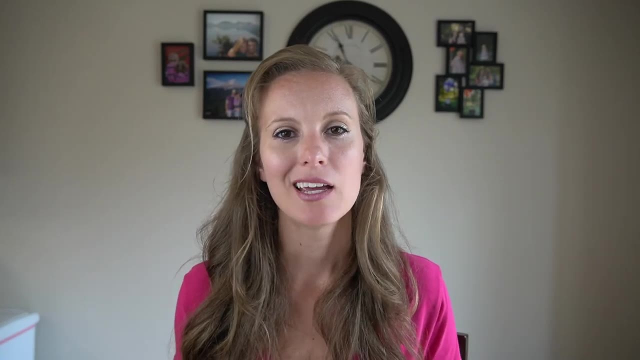 pile of clean clothes that need to be folded and put away, And it's just overwhelming and exhausting to even think about taking care of that much laundry. Doing one load on each weekday is much easier to maintain than trying to do all of your laundry on one day of the week, But be sure to 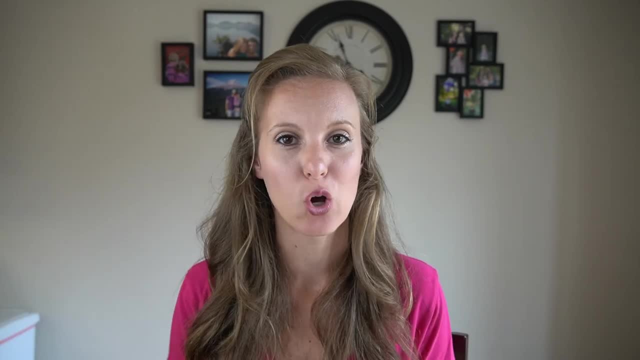 check out that article that I linked down below for all 12 tips on creating your own laundry routine. The third thing to remember when creating your own laundry routine is to keep your laundry clean. The first thing that people who always have clean houses do is they keep their kitchen clean. 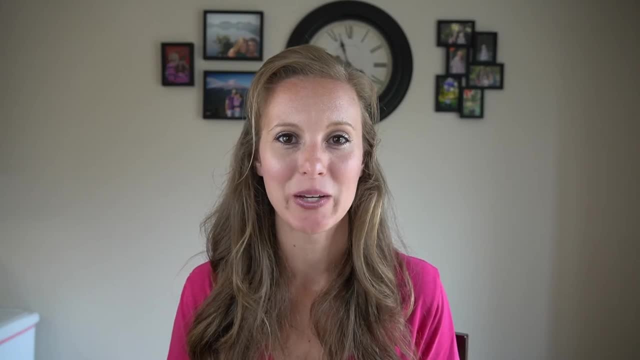 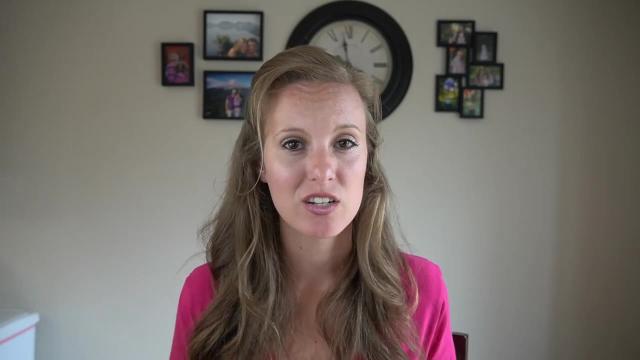 throughout the day. If you want to have a house that feels clean when you walk into it, keep your kitchen clean. Nothing else makes your house feel more dirty than a kitchen that is out of control And, depending on where your kitchen is located in your house, it can be really obvious to your 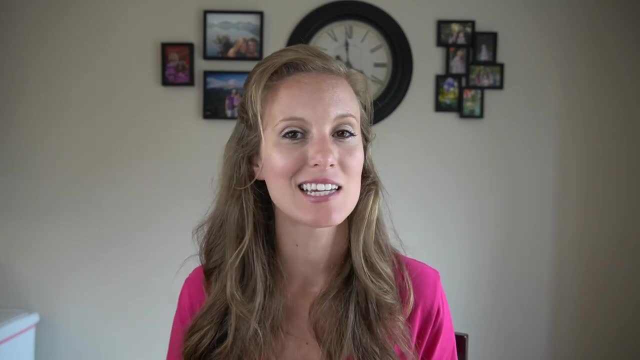 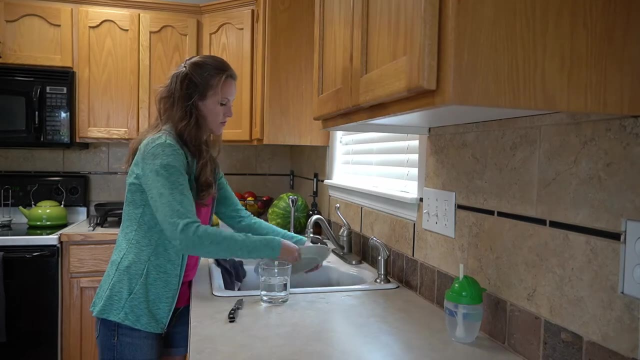 guests when your kitchen is a mess. Now, keeping your kitchen clean doesn't just mean that you clean it at the end of each night. It means that you clean it after every meal. It takes so much less time to clean your dishes right away than if you wait to do it later. 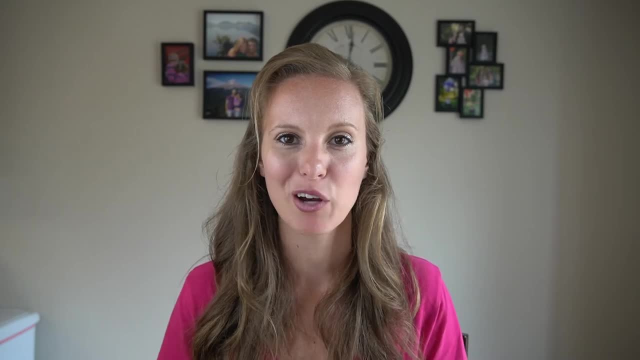 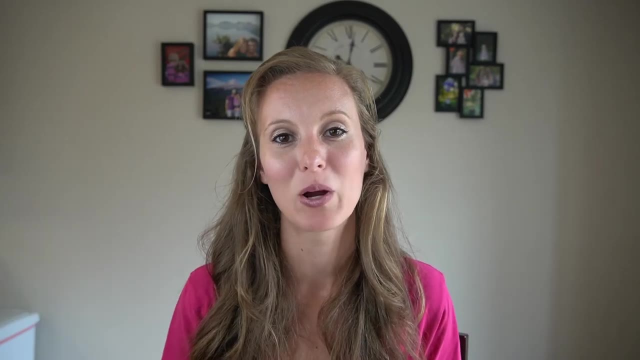 If you'd like a step-by-step guide for the fastest way to clean your kitchen after every meal, check out this video here for more details, And I will also leave a link in the description down below with the busy mom's guide for cleaning your kitchen the easy way. The fourth secret to always. 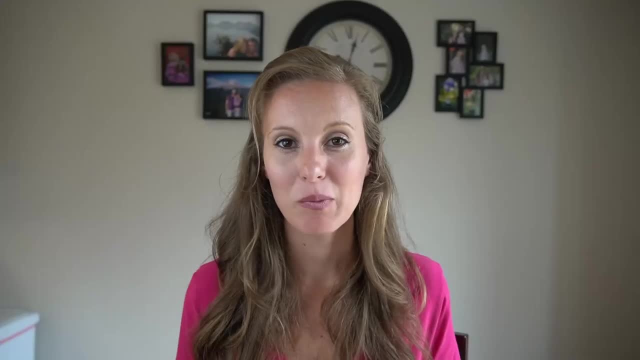 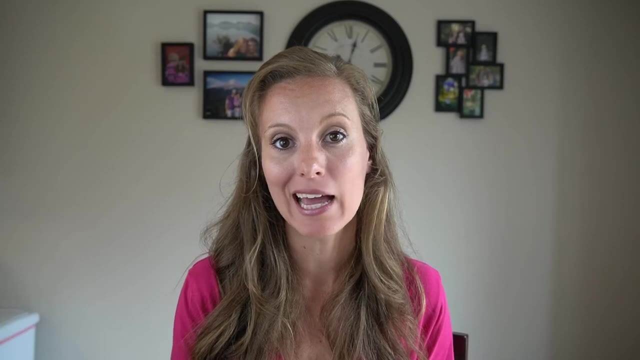 having a clean house is to have a weekly cleaning routine. People who have clean houses all the time don't clean their entire house every day, but they also don't just clean their house once a week and expect for it to stay clean all throughout the week. Instead, they have a simple weekly cleaning. 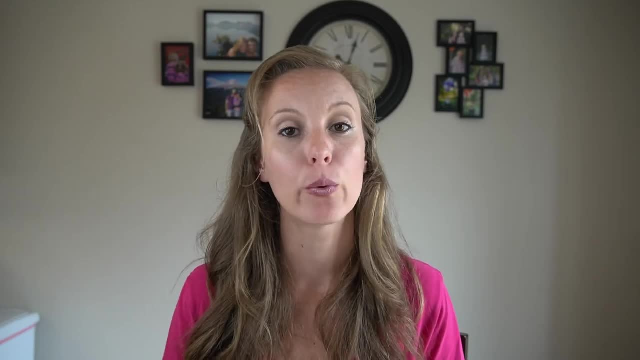 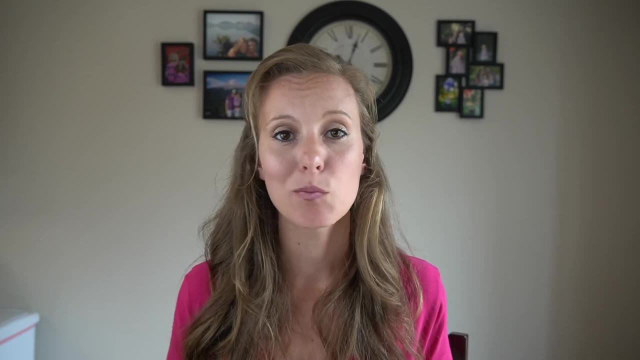 routine that helps them get all of their cleaning done throughout the week. This makes cleaning a habit and it also keeps them from getting burned out from cleaning all the time. A simple weekly cleaning routine shouldn't take you any more than 20 to 30 minutes to complete every day. 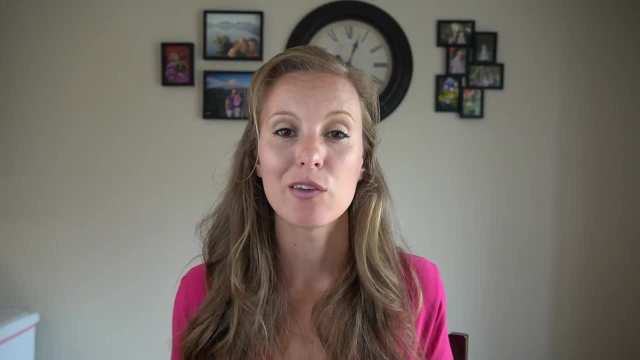 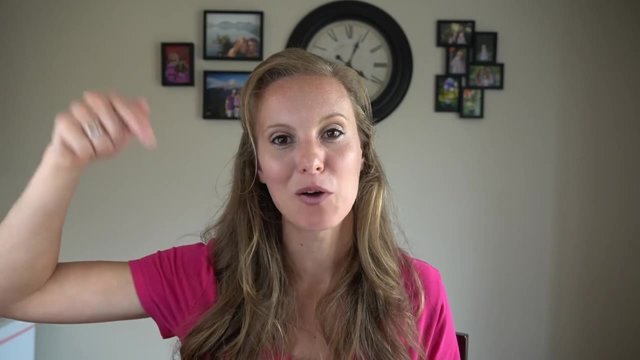 but it will keep your house clean all throughout the week. If you'd like to see my simple cleaning routine and how to create your own, you can check out this video here, and I will also leave a template down below that will walk you through how to create your own weekly cleaning routine. 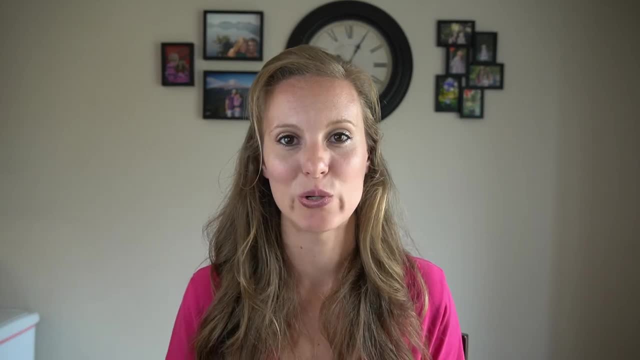 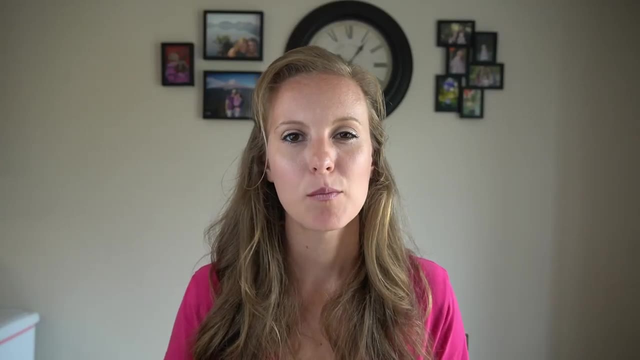 The fifth thing that people who always have clean houses do is they set aside time each day for cleaning. Having a small amount of time set aside every day to clean makes sure that all the cleaning gets done every week without needing to spend all of your time cleaning While the specific time 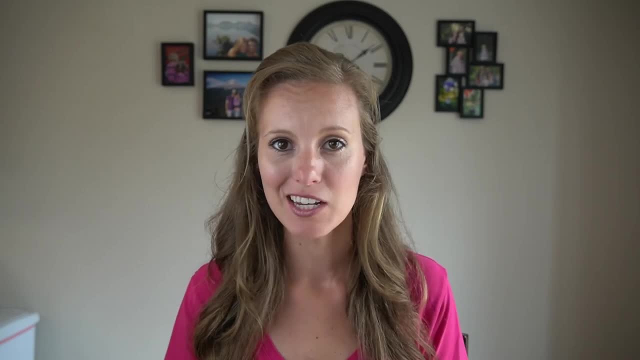 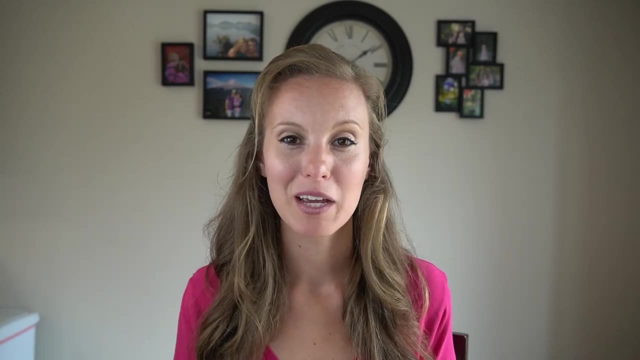 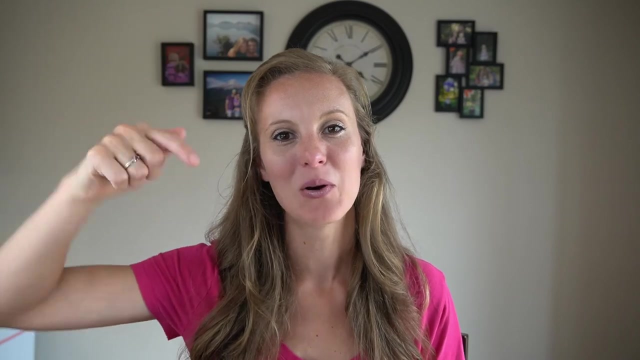 that you decide to clean every day will probably be different than when I do. the best way to make sure that you have the time set aside is to create a simple block schedule, And if you'd like more time for that, check out this video here, and I will also leave a template down below that will. 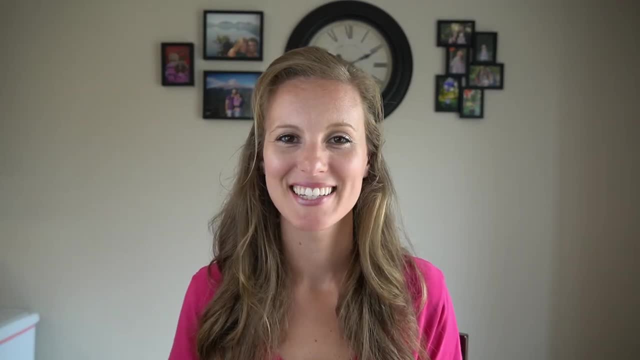 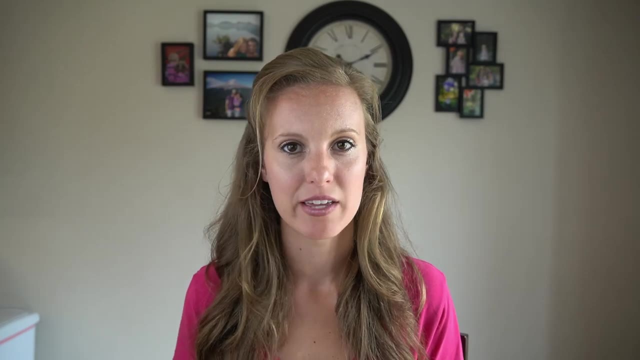 help you customize and create your own block schedule. Number six: people who always have clean houses get rid of their clutter. The biggest thing that you can do to make your house feel clean all the time is to declutter it. Only having things in your home that you love or use on a 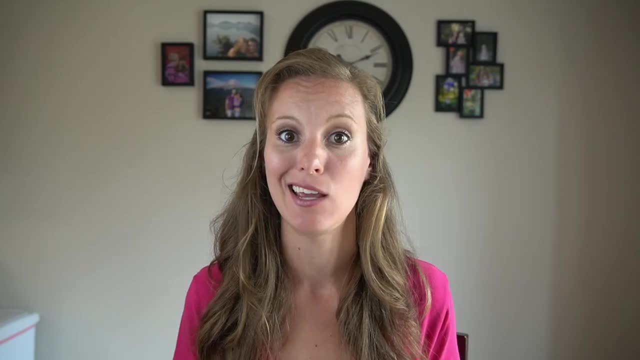 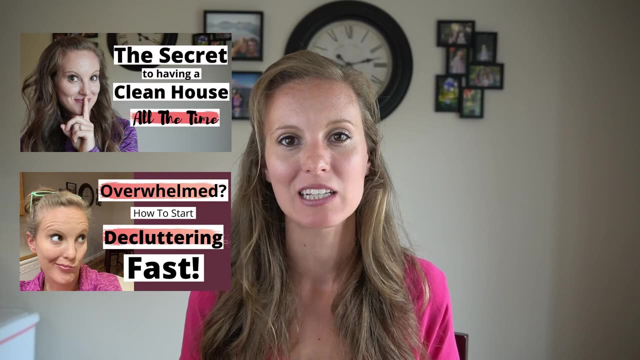 consistent basis will make your house feel clean and tidy all the time. If you think that decluttering would help your house feel cleaner all the time, I have a couple videos about how to get started with decluttering and I will leave both of those down in the description below or you can check. 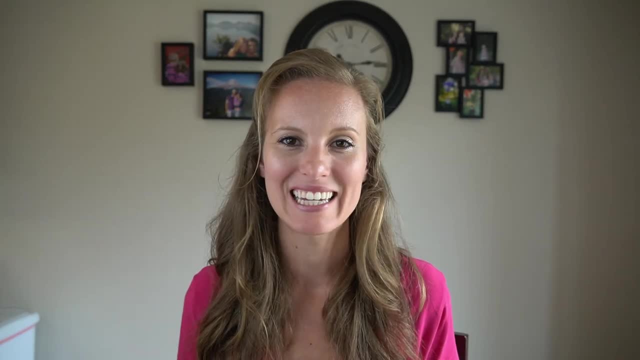 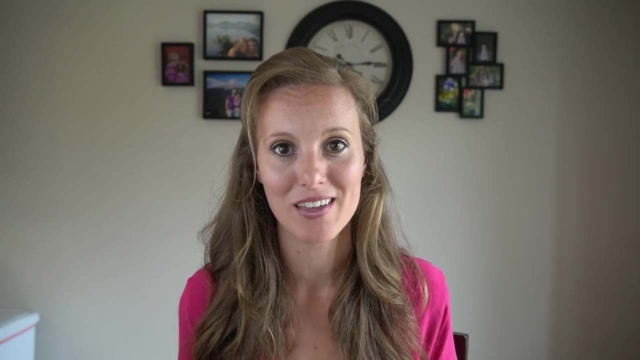 out this video right here. The seventh trick to always having a clean house is to put things back when you're done with them. One of the fastest ways to make your house feel dirty is to just leave things where they are when you are done with them. Putting things away right away will save you. 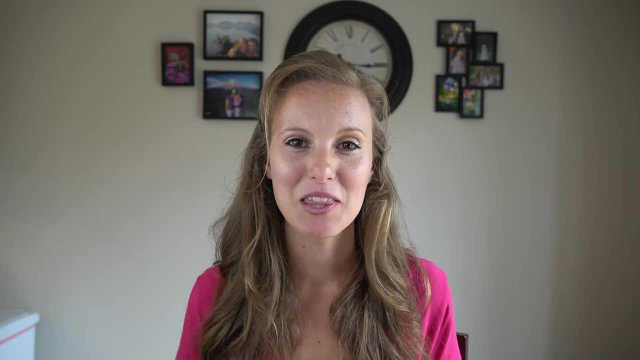 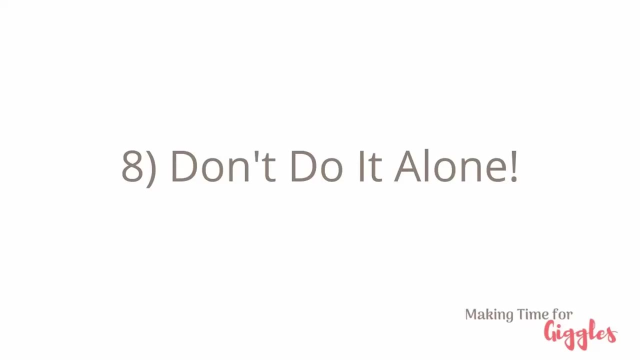 time and energy when it's time to clean. And if you've stuck with me this far, I have a bonus tip for you. The eighth secret that people who have clean homes all the time know is that they don't do it alone. People who have clean homes all the time know that they don't do it alone. People who 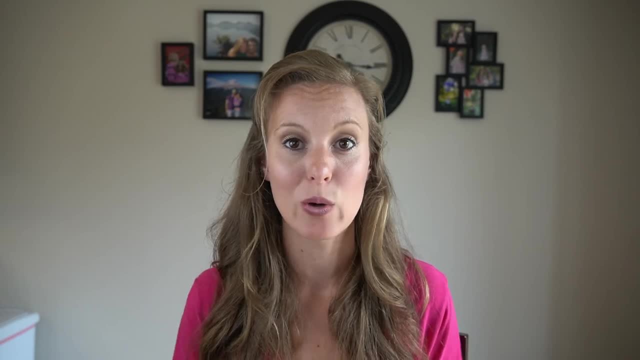 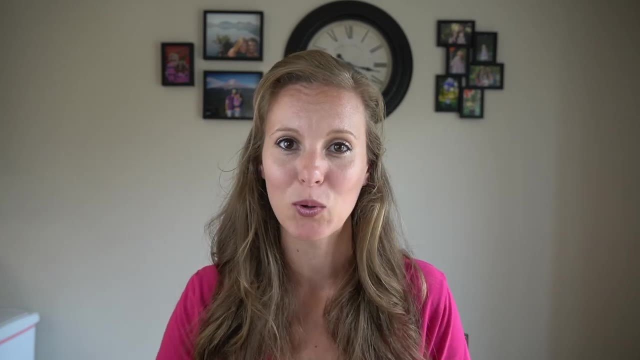 have clean houses all the time, enlist everyone else in their house to help out. At least that's how I do it in my house. Since I'm not the only one making the mess, it doesn't make sense to me that I should be the only one cleaning up If you and your spouse are both working outside the home.